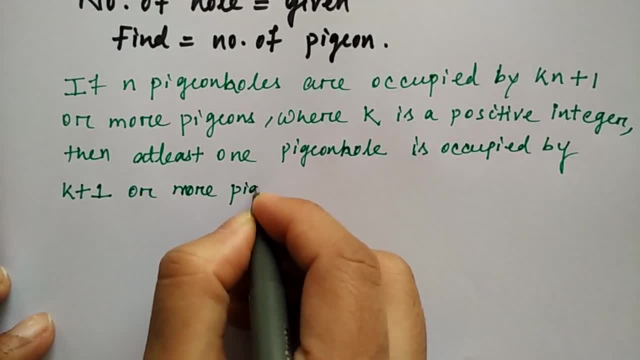 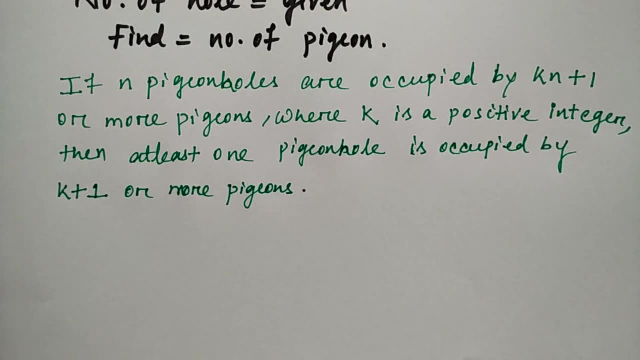 more regions. so the meaning of this definition is for n. if n peasants are occupied by K into n plus 1 or more peasants, then K is a positive number. and for all, this condition just to satisfy that at least one peasant hole is occupied by K plus 1 or more peasants. so we'll see the examples, how to solve this. 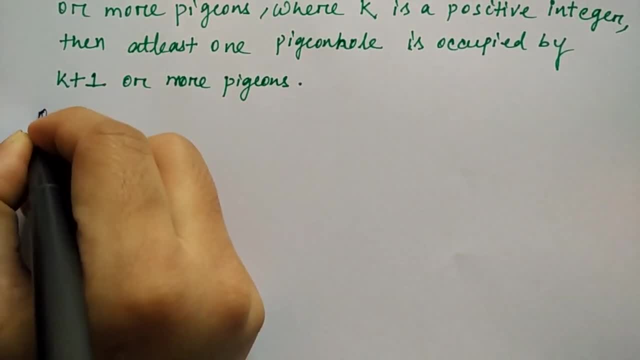 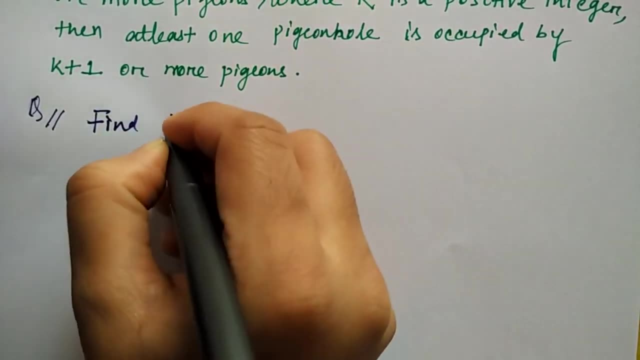 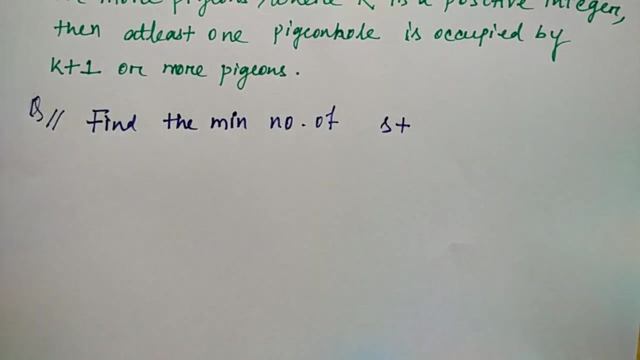 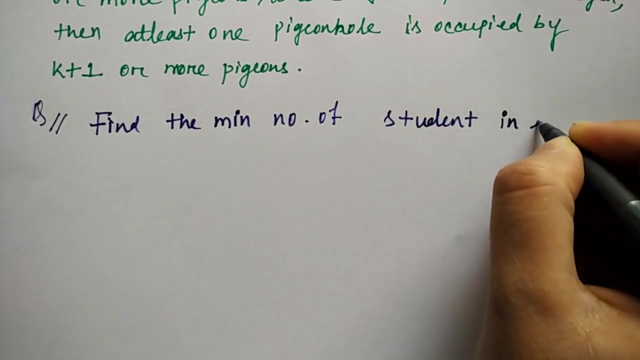 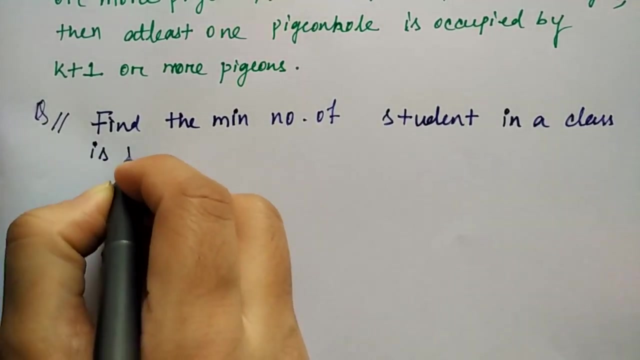 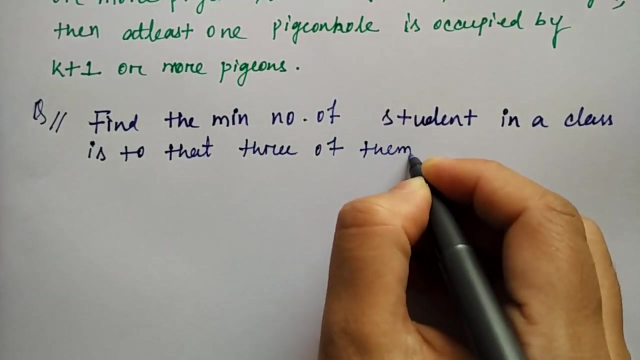 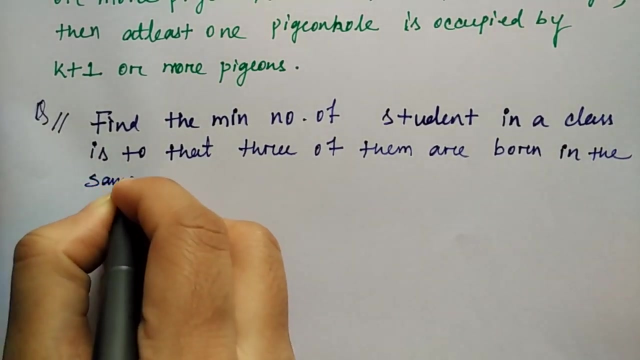 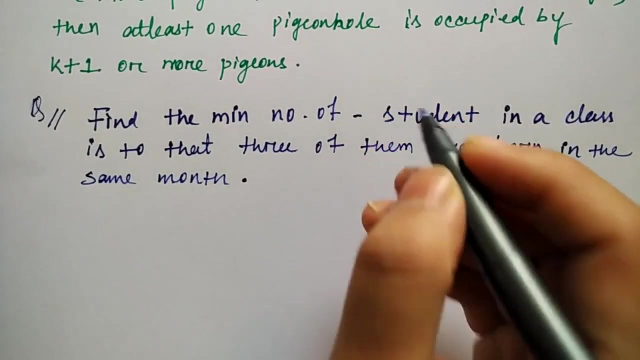 there is a question: find the minimum number of student in a class is to be that three of them are born in the same month. so it is asking that the total number of student or minimum number of student in the class you have to find out so that at least three of them are born in the same month. so 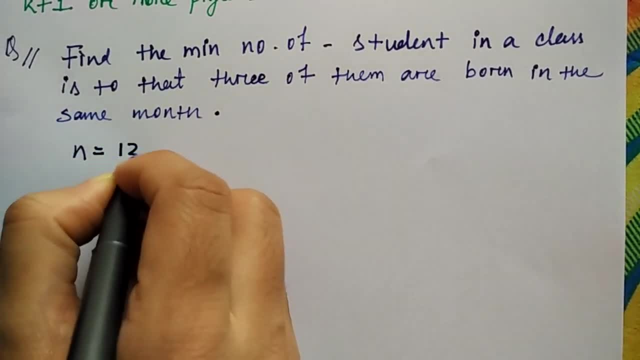 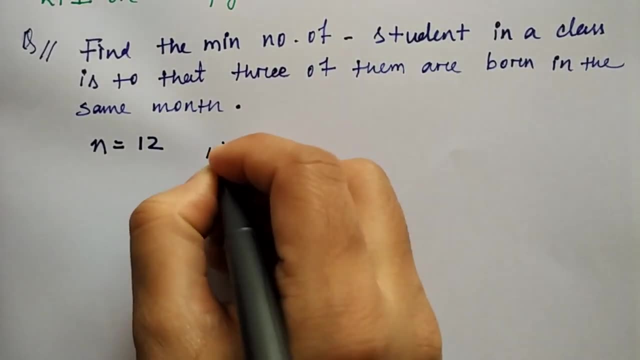 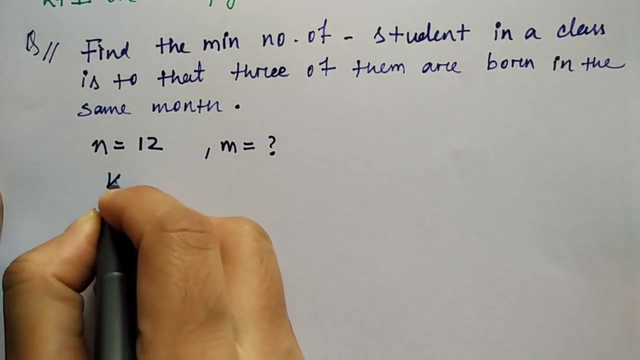 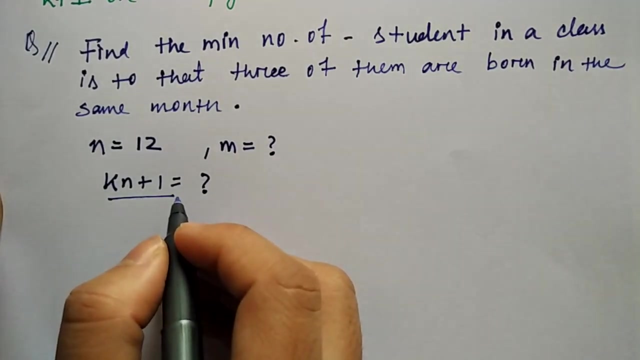 totally. how many months are there? there number of months are equal to 12, so that will be obviously n. that is a container and we have to find out the object, that, we have to find out the m value. so n value we have already got. and what is k? n plus 1? we should try to understand now. okay, what is k? n plus 1? it is the condition. 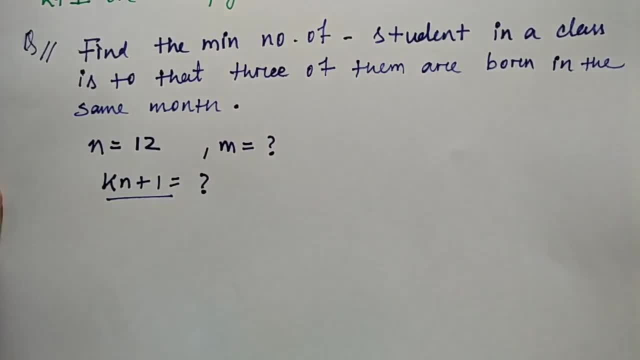 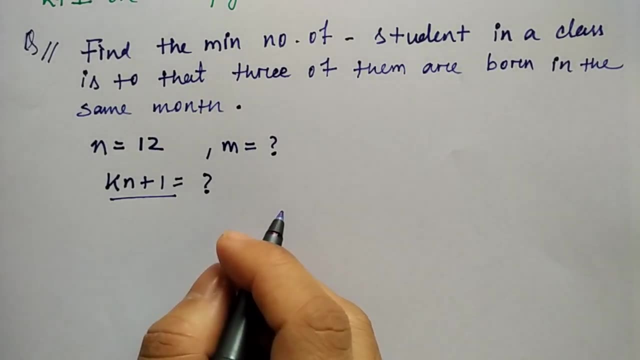 or the what you say, the property according to which we have allocated the peasants into the pigeonhole. so it has told that, um, at least three of them are born in the same month. so, whatever the specific condition given, that is always taken as the k? n plus 1, so that is, k n plus 1 is given. 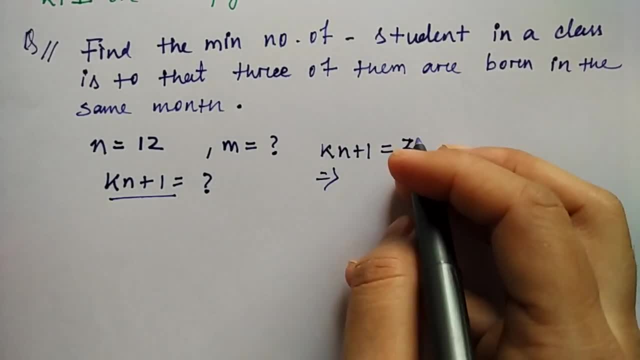 as 3. so what will be k of n here? k n plus 1 is given as 3, so that is k n plus 1 is given as 3. so what will be k of n here? so that is, k n plus 1 is given as 3. so what will be k of n here? 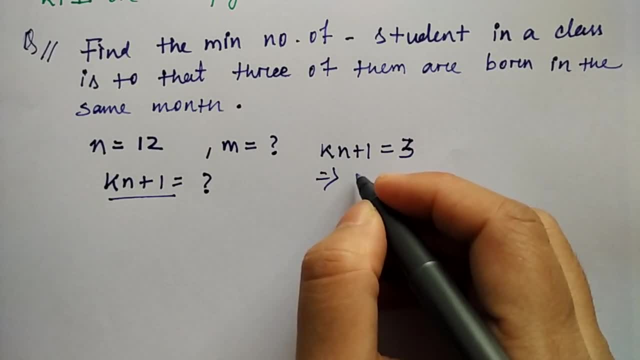 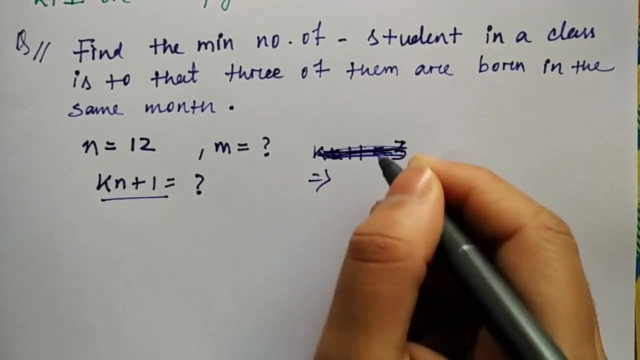 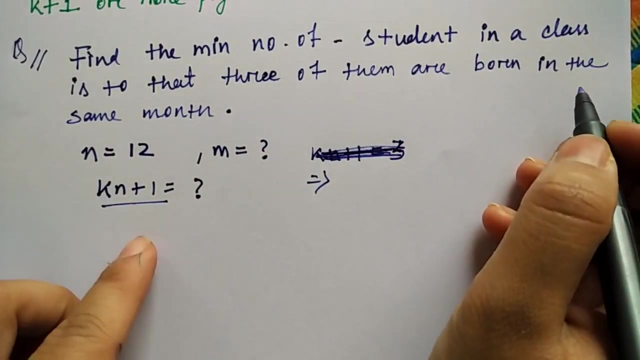 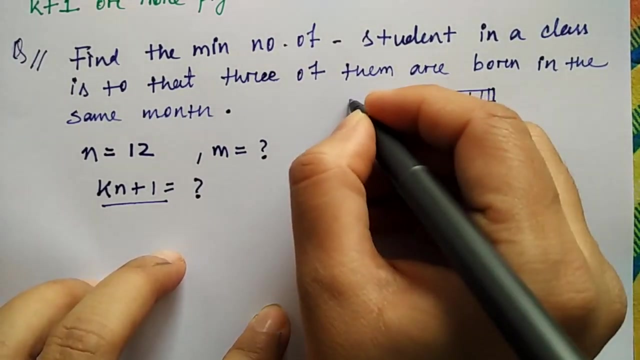 sorry, like this thing we have to determine, but this part is wrong. see what is the special condition given here is three of them are born in the same month. it means if the box has some 12 number of value, in one box you should have three or more student right and according to. 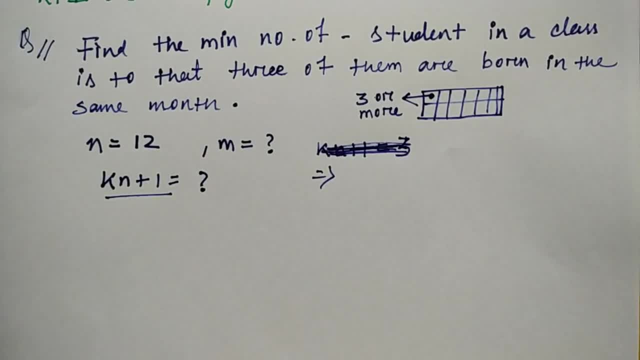 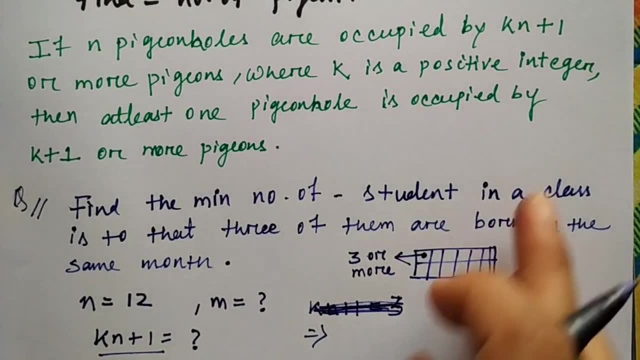 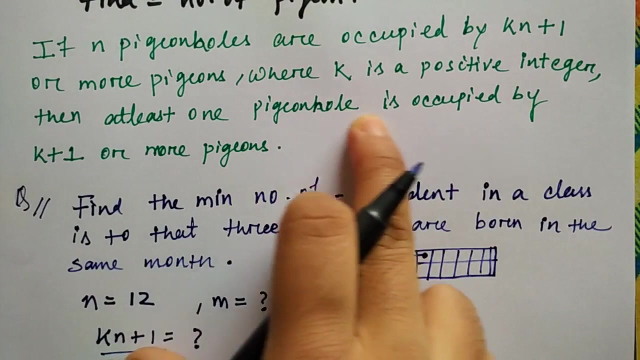 the definition of the generalized pigeonhole principle what it is, given that if you have n pigeon occupied by k plus 1 or more pigeon, so here occupied by k, k, n plus 1 or more pigeon, where k is a positive number, then at least one pigeonhole is occupied by k plus 1 or more pigeon. 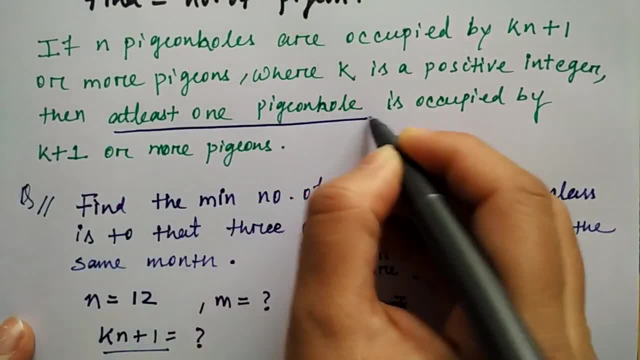 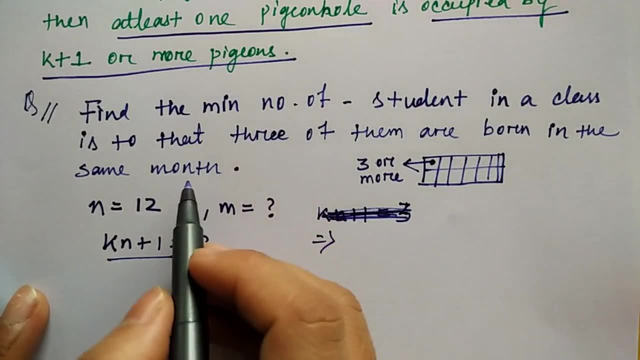 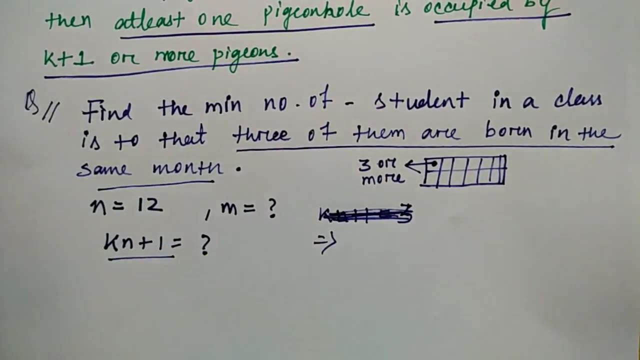 so what is the most important thing given here, at least one pigeonhole is occupied by k plus 1 or more pigeon, and if you see the question, what it has told that in a class is to that three or three of them are born in the same month. in me it means 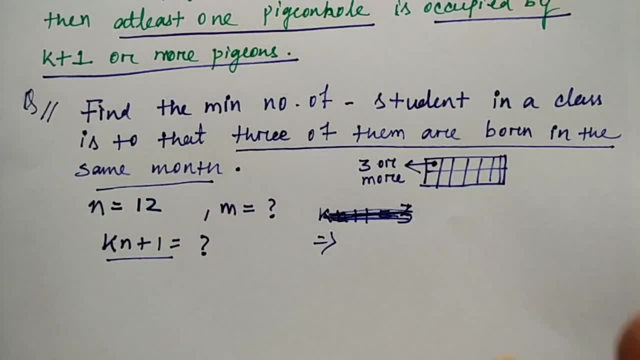 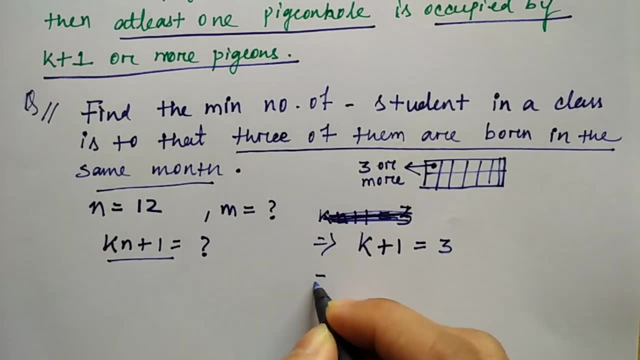 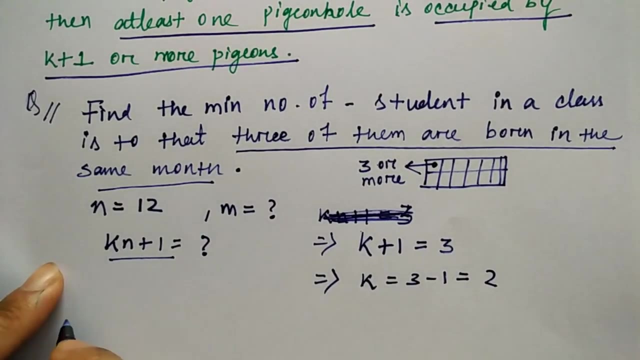 out of the 12 month, in one month three are born. it means this place is like: according to the definition, it is k plus 1 is having three students. so k will be equal to 3 minus 1 into 2. now we have got the variable k, so what will be the object? that is, m equal to k, n plus 1. 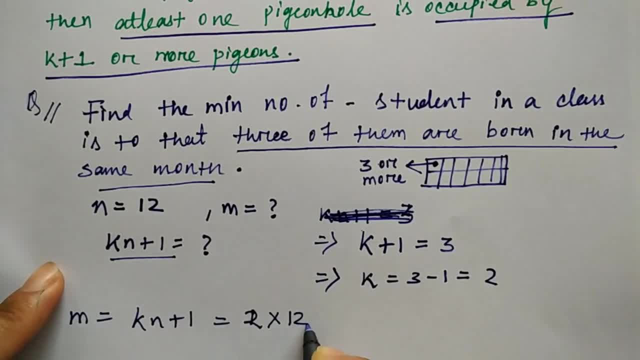 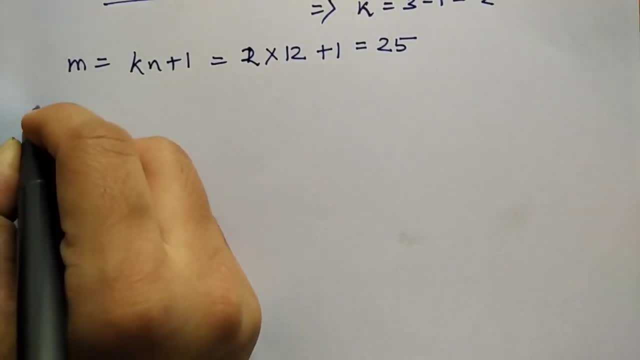 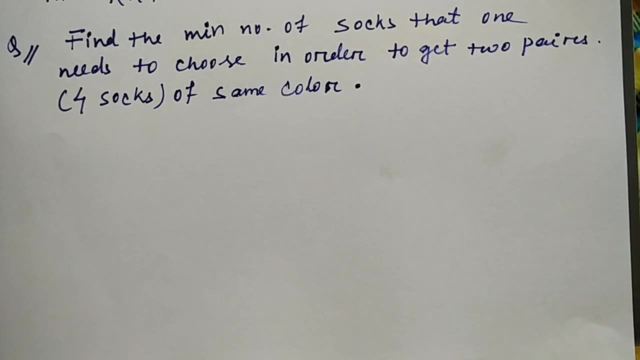 that will be equal to 2 into 12 plus 1, that is 25. so this is the answer and solve one more question to make it more clear. so here is this question. it is saying that there are three different kinds of socks, that is, red, white and blue in color, and you have to determine the. 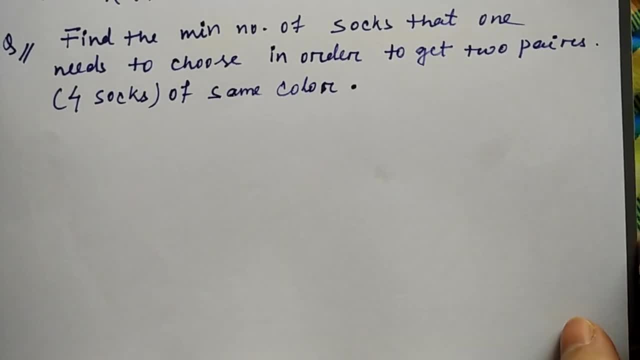 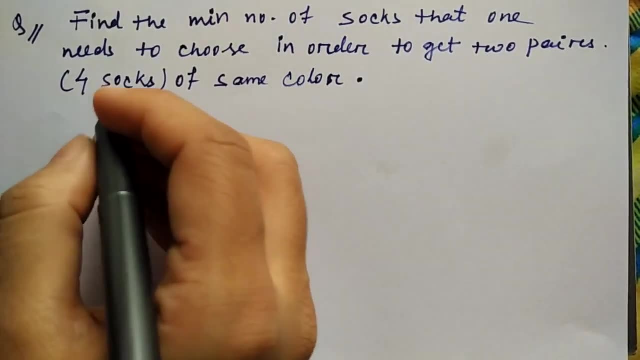 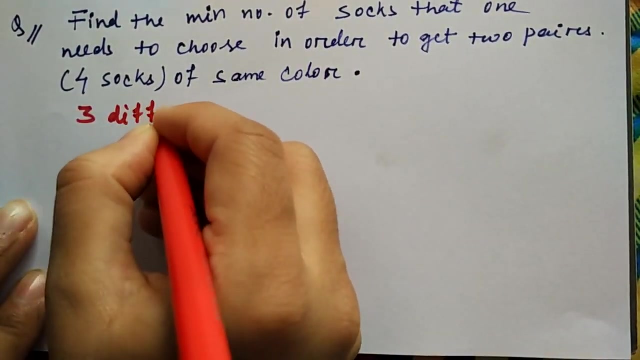 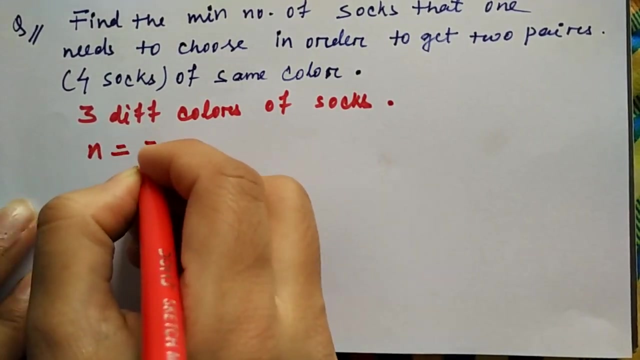 number of socks that one need to choose in order to get two pair, that is, four socks of same color. so first of all, three different type of socks, are there? three different colors, three different colors of socks. so already there, it means n equal to 3. that is the container. you can say right, like how, how,